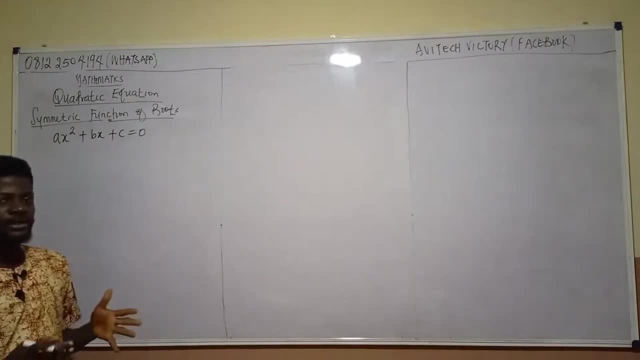 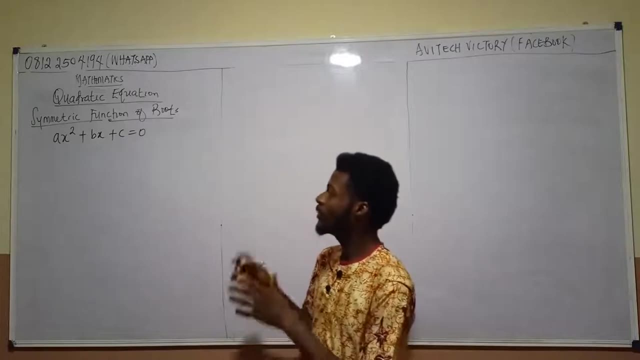 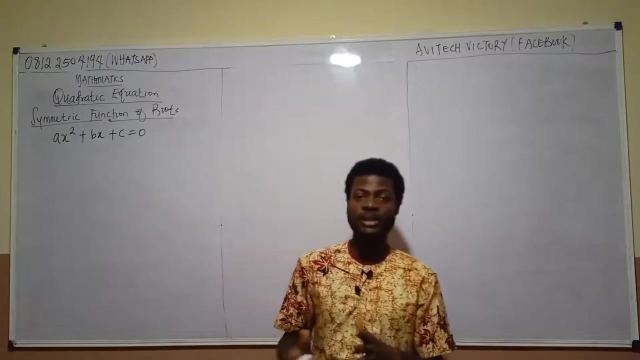 So majority of us have already seen that very formula before. So we have, as squared plus bx plus c, equal to zero. Now I want to just treat symmetric functions of roots. Now, what are roots Basically? let me use a layman language. 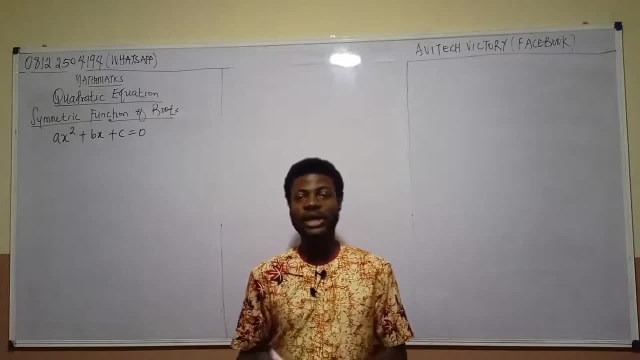 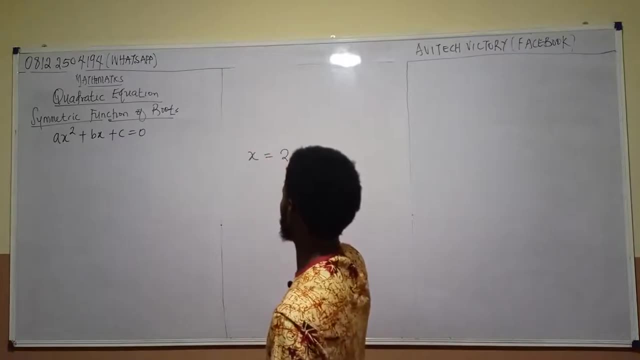 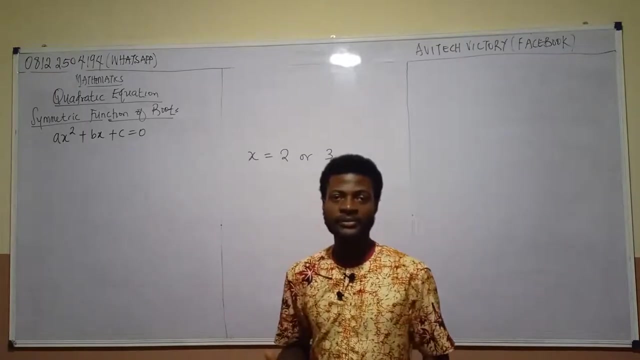 The answer you get after solving an equation is called the roots of that equation. So that means, if I don't solve an equation and you got s equal to or 3.. It means 2 and 3 are the roots. That's the meaning. It means 2 and 3 are the roots. 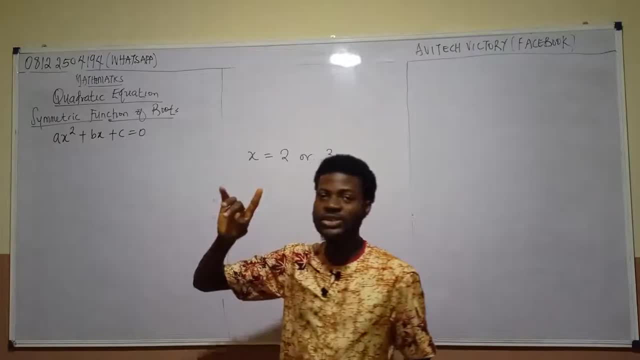 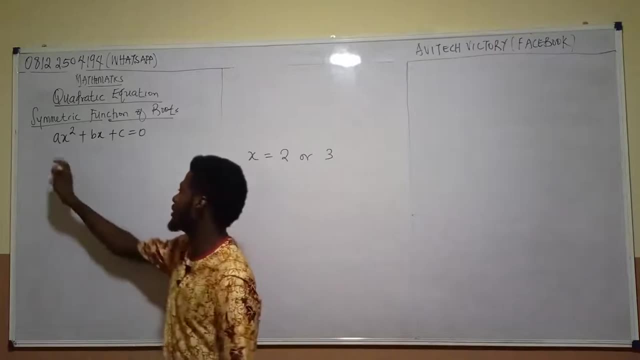 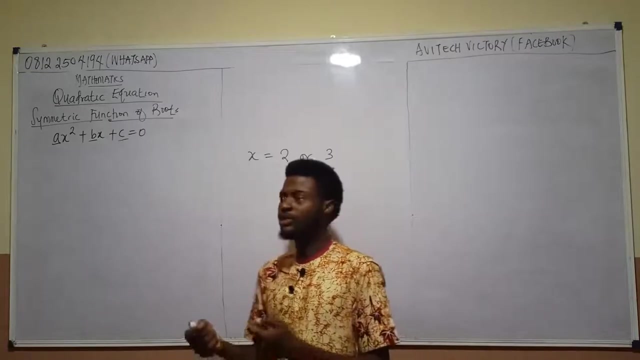 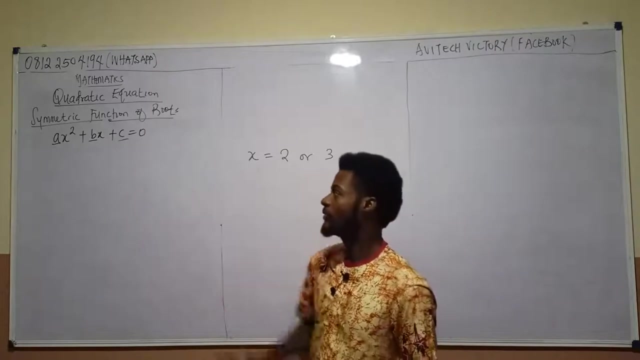 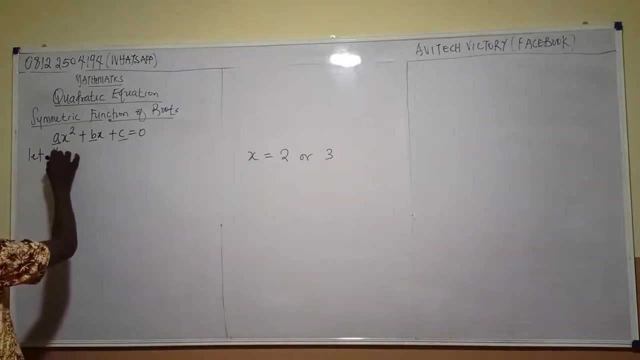 Now the symmetric function of roots is actually discussing relationship of the roots and these coefficients- a, b and c. That's what symmetric function of roots is all about. It's the study of relationship between these roots and The coefficients. Now let us make our first proposal here. So let the roots be alpha and beta. 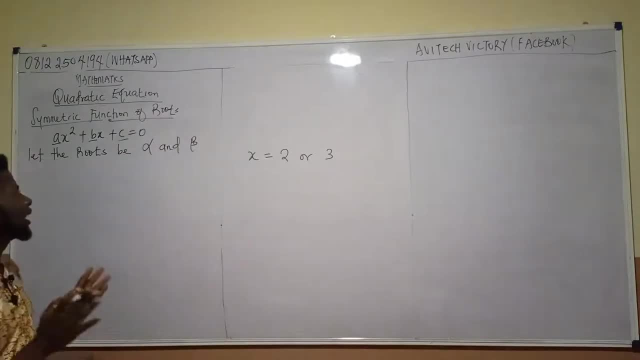 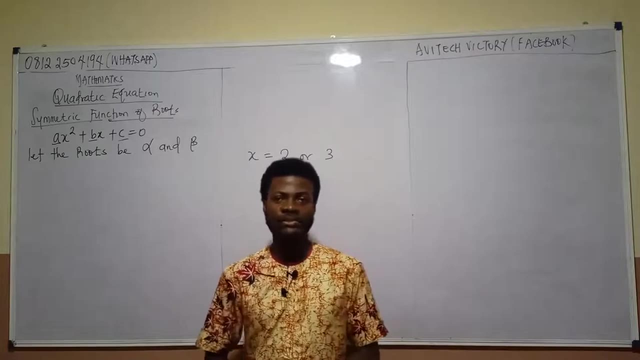 That's the first thing you do. Let the roots be alpha and beta. Now, mind you, we can just. I would have just written the formula down, But let me just quickly derive it so that we move ahead. I'll just quickly derive it so that we move what? 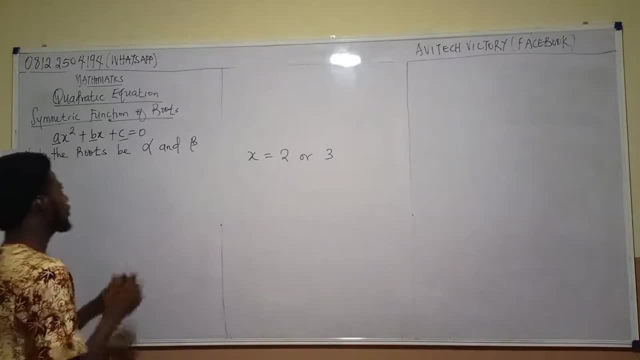 I'll just quickly derive it so that we move ahead Now. first of all, look at this. Look at this. Remember that if we want to find an equation, if we want to derive equality equation, what do we do? We'll say: x squared minus sum of roots. close bracket. x plus product of roots. 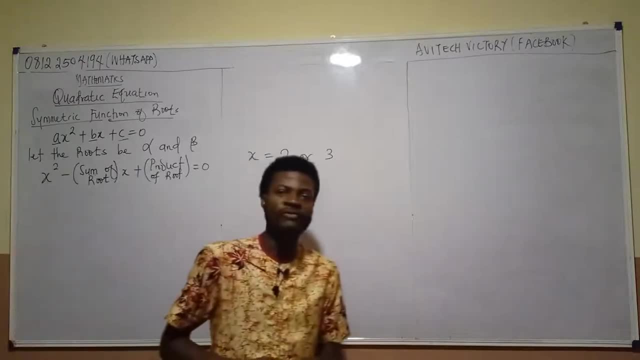 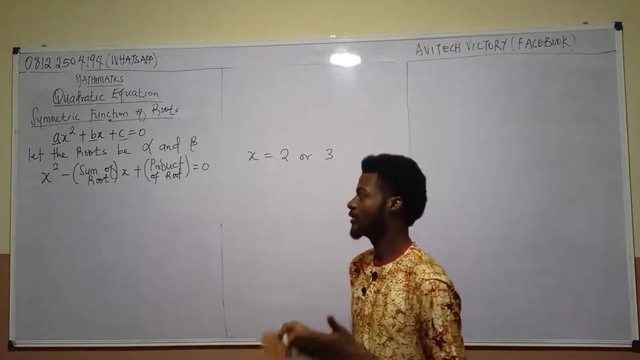 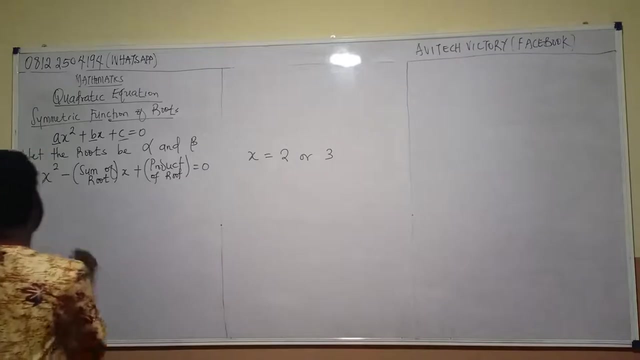 I don't know if you can remember, I don't know if you can remember want to find an equation. what do we do? we use this very formula: s squared minus sum of roots, bracket s plus plot of roots. so let us proceed, and this will now become s squared. 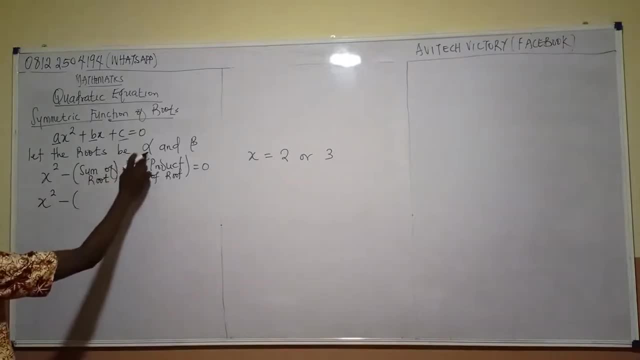 minus what do we say? the roots are alpha and beta. so that means the sum will now become alpha plus beta. then close bracket. you put your what, you put your x, then plus what would the product become? alpha, beta. equal to what? zero? now there's nothing you can do here. you can't do anything here. 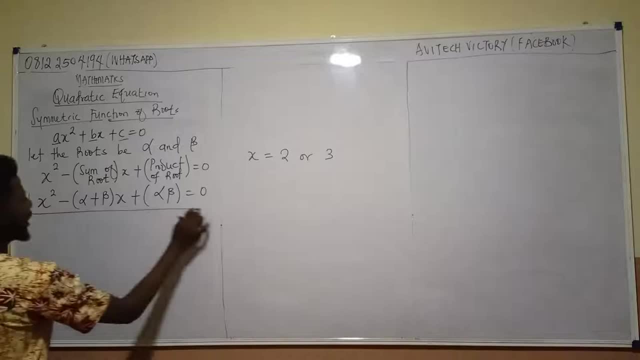 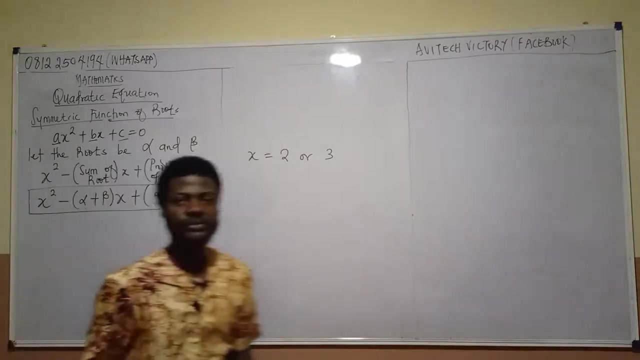 so i'm going to keep this expression somewhere in my mind. we're going to come back to it. so this is s squared minus alpha, plus beta, plus alpha beta. now, remember, this is the roots. this equation using what the roots, this equation using the roots. remember we said symmetric function is relationship. 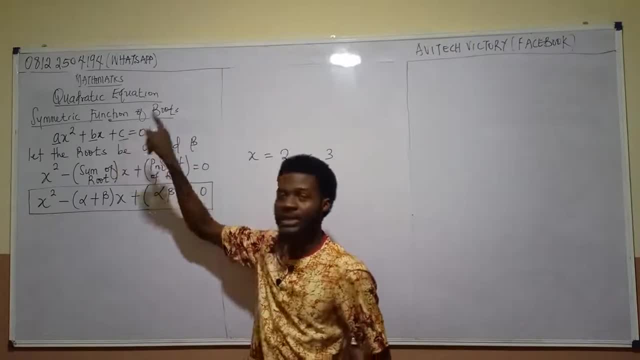 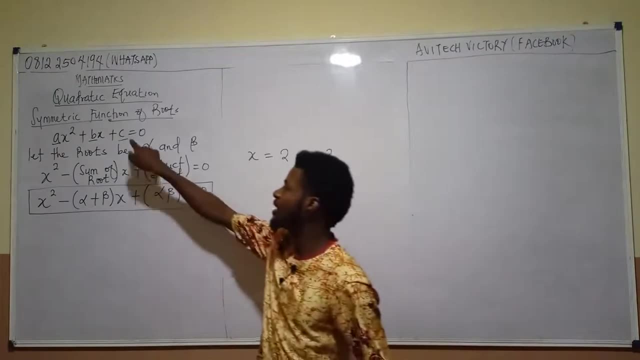 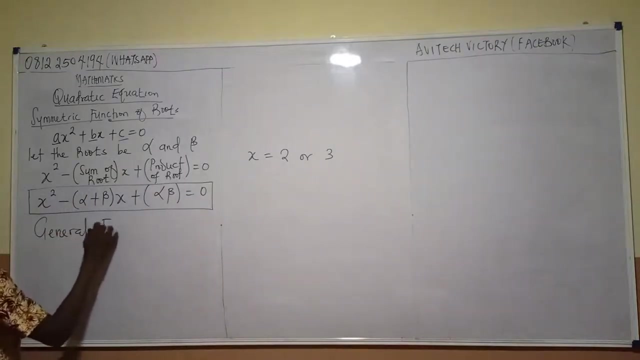 between the roots and this: a, b and c. so right now we've gotten an equation using what the roots. now, what is the general format for the equation, the general format, the general form? the general form is a s squared plus bx plus c, equal to zero. now, if we're trying to compare these two, because right now we're finding 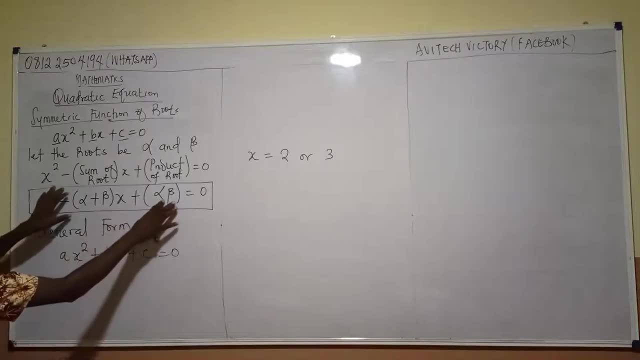 the relationship between the expression that has the roots and the general form. so that's what we're trying to do. so let's try to make this expression look exactly like this by doing just one thing. and what is that thing? if you can see, here s squared, s squared, there's no number in front of. 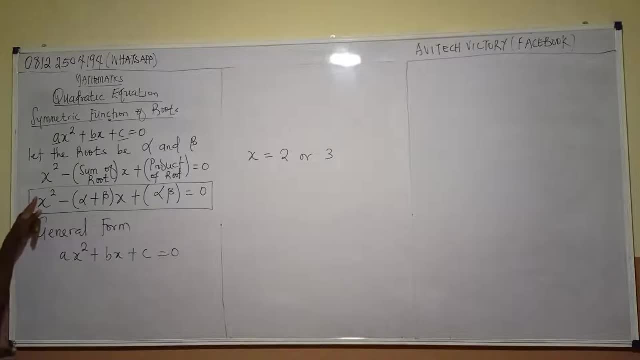 it, or rather we have one in front of it. so what do we do? we're going to do is we're going to do a general form. so what do we do to make this part become only one? because the general form has a general form has a. so what do we do to now make it one, so that the two of them will look alike? 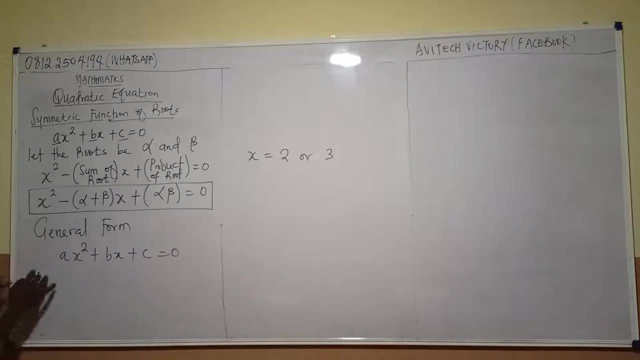 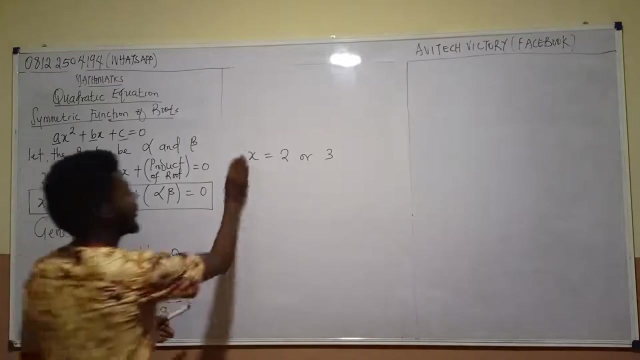 so what i will say is, since i have a here to remove a, i will say: divide by a. so that means i'll have a s squared over a plus bx over a plus c, over a equal to zero. so the next thing i'll do is a and a can cancel. so that will leave me with a and a can cancel. 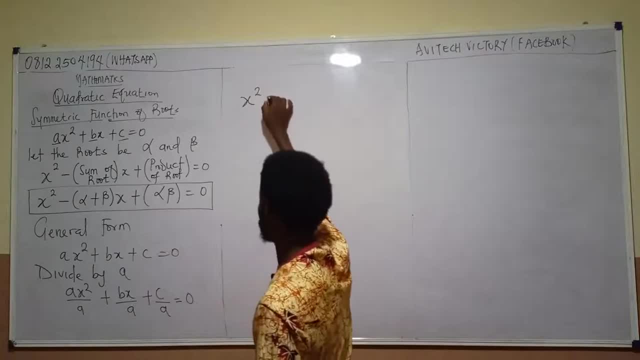 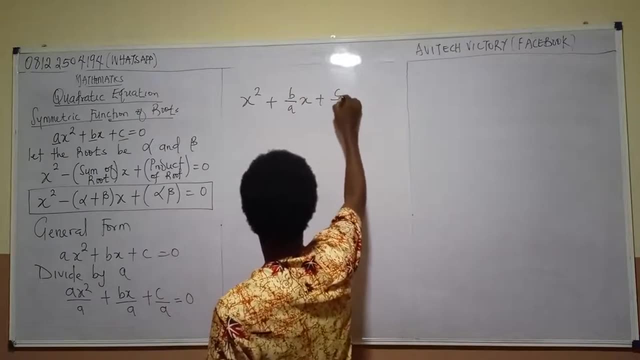 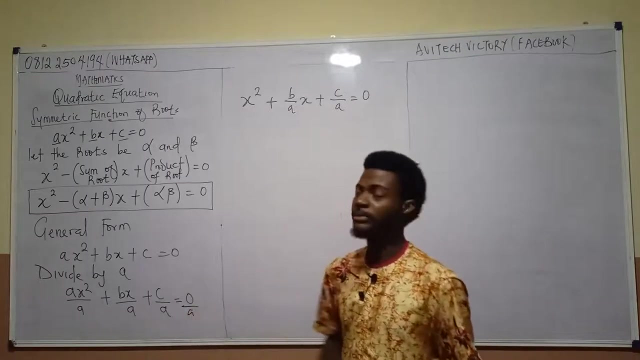 so that will leave me with s squared. then, plus this is b over a, b over a, x plus c over a. equal to what zero, though? i would have said zero over a, but zero over a is still same thing. now, this is what i didn't have, so these two equations are going to be equal to zero over a, so i'm going to. 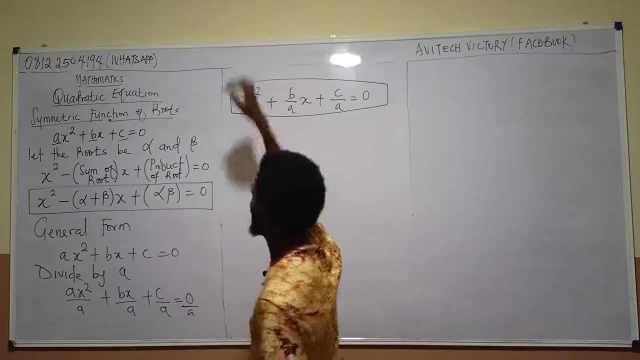 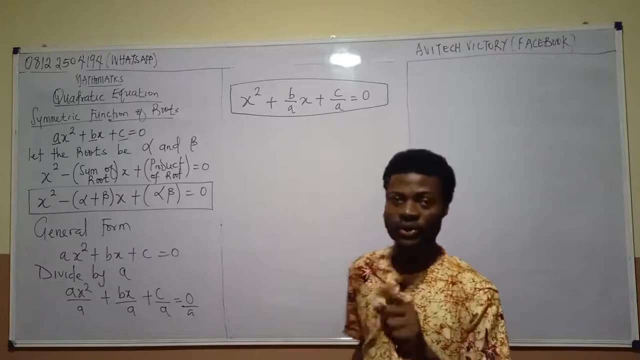 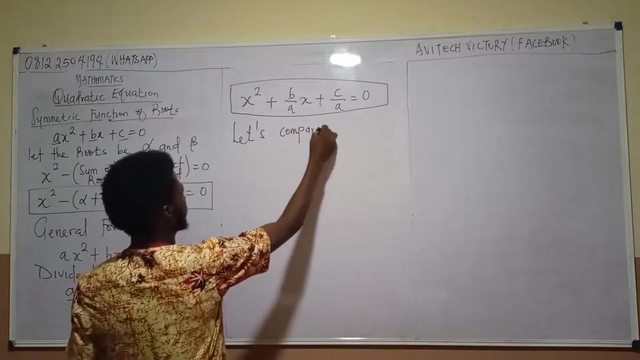 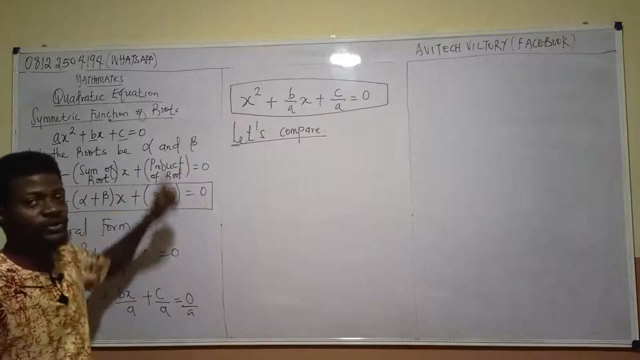 have two equations, so i have two equations. now i have two equations, this and this. the next thing i'll do is to compare them. the next thing i'll do is to compare them. so let's compare, let's compare. so look at this: this is s squared and this is s squared. they'll both cancel themselves, so it's. 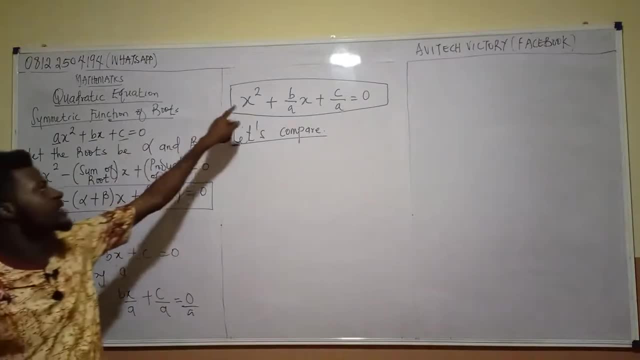 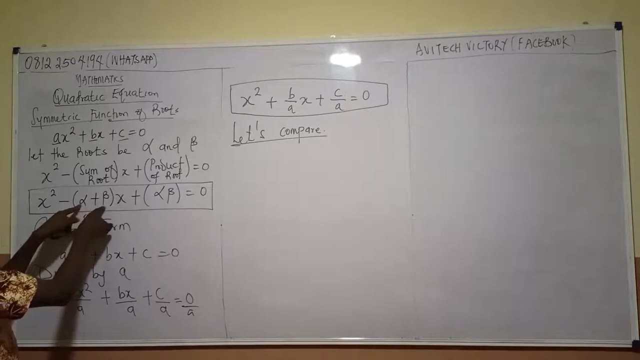 gone. look at it, this is s squared and this is s squared. they'll both cancel and that will be all. so they will go now. the next thing is: i have alpha plus beta bracket x. here i have beta over a bracket x. so, as you can see, this is x and this is x. i'm comparing the two. 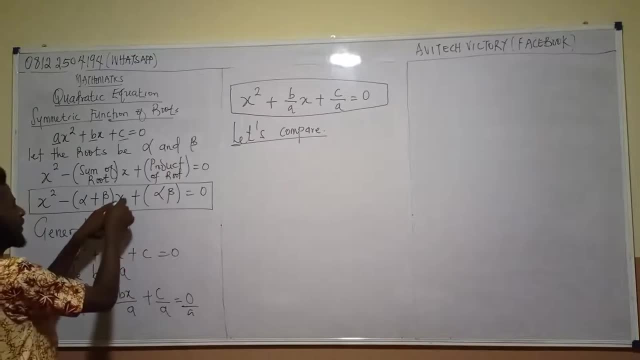 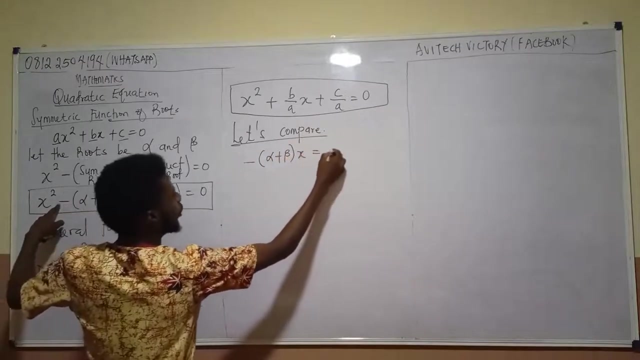 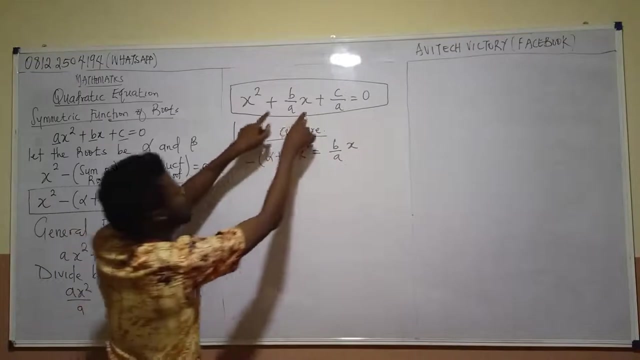 they have the same coefficient. i have x here and i have x here. so if this s should take away this s, it means i'm having minus. this is a minus and so you have to be careful. minus alpha plus beta x equal b over a x. are you getting the phenomenon? this part has x. i compare with the part that has. 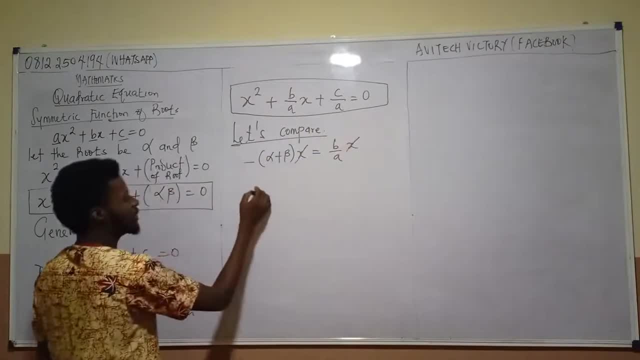 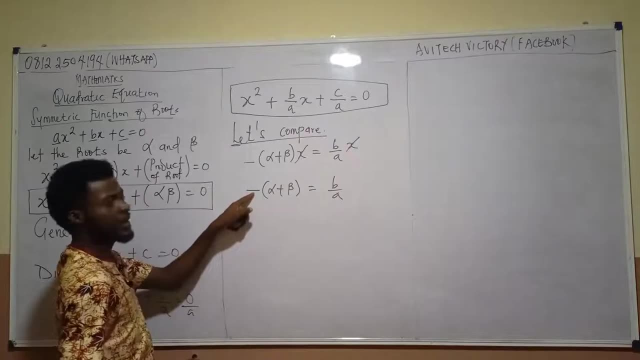 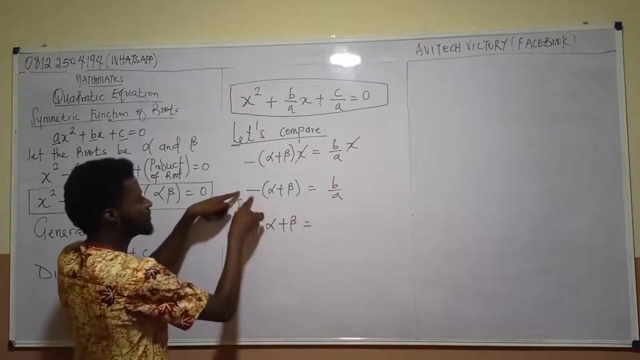 x. so if s should take away x, i'm left with minus alpha plus beta equal b over a. now, definitely this minus. it should not be here. let me just take the minus to the other side. so that means alpha plus beta is equal. if this minus should come here, we have minus b over a. so what does? 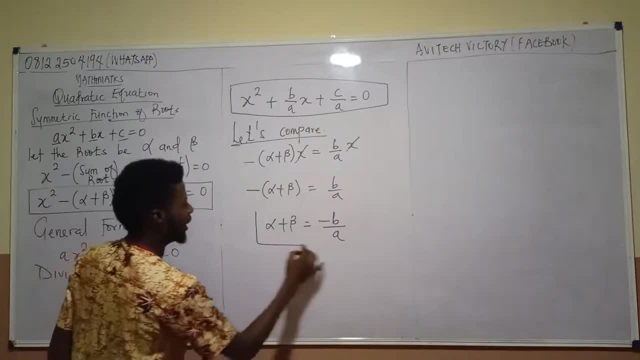 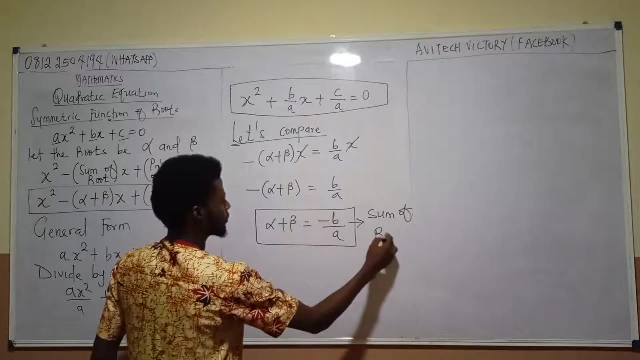 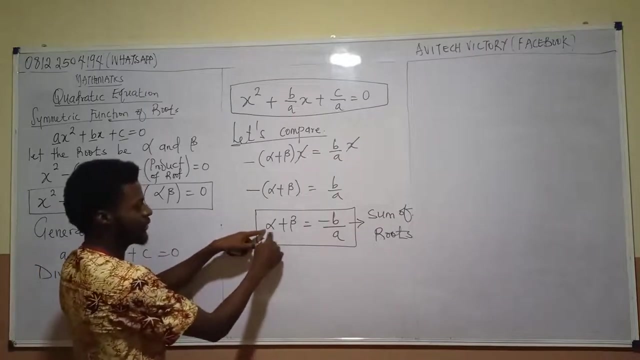 that mean? that means this is the first formula for sum of what roots? sum of roots, that's the first formula. so what this means? as you can see, these are the roots, these are the roots and these are the coefficients. so this very formula is a relationship showing that the sum 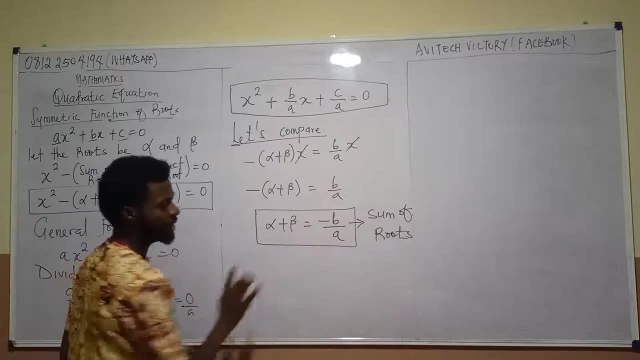 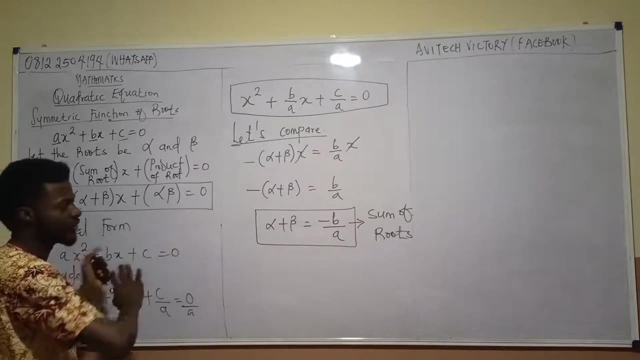 of the roots is equal minus b over what a. so this is the first thing. you might not listen. it's not a must for you to know the derivation. it's not a must for you to know the derivation. but please, this should not leave you. it should not leave you. nine day, important pass. 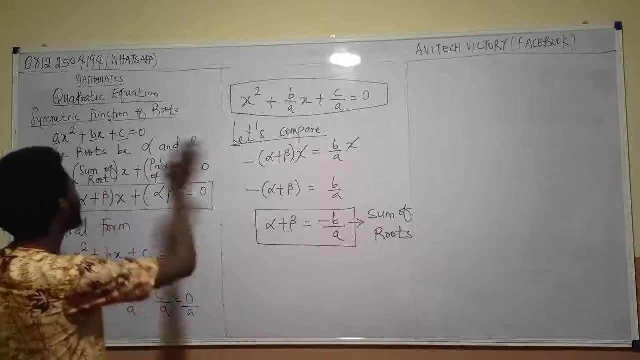 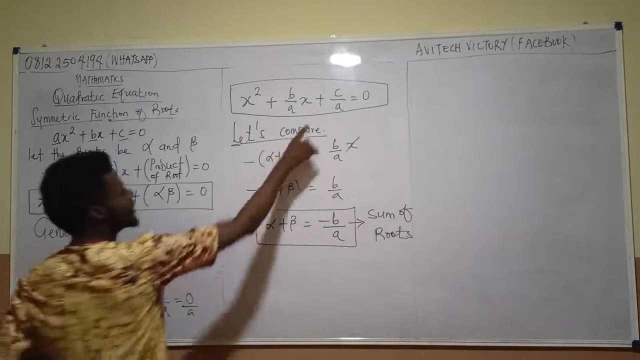 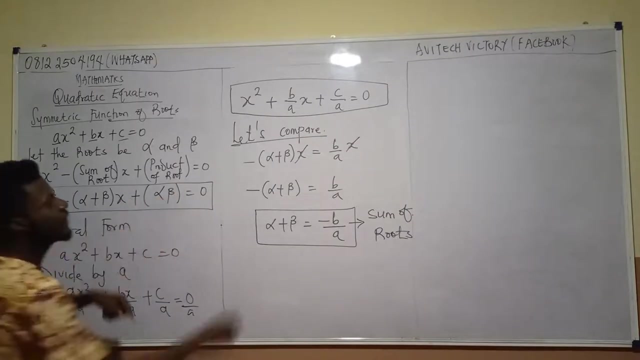 it as in it didn't have all these ones. you might not even need it safe, is this one that day more important now? let us continue now. the next thing is this: c over a. look at this part. this part is plus alpha beta. there's no number, there's no alphabet here. this is c over a, there's no other. 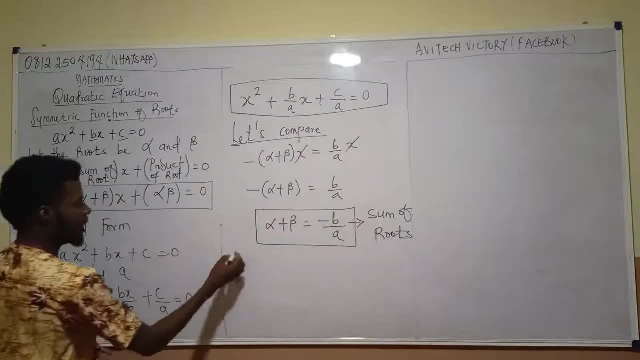 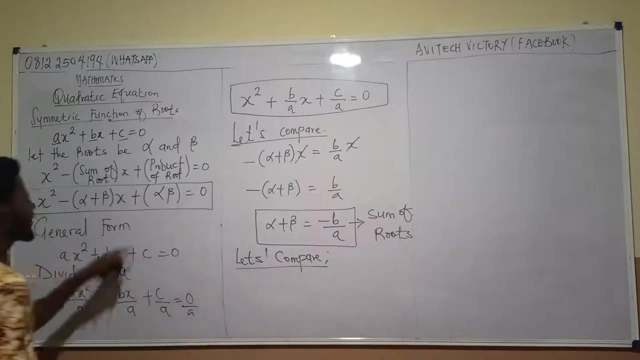 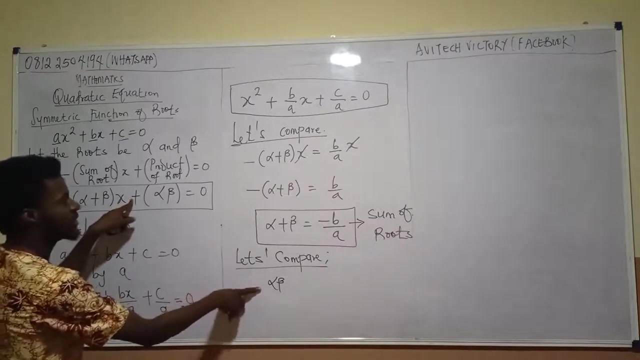 so can we compare them? yes, we can compare them. so let's compare again. let's compare again. so that means i'll be having: this is alpha beta. this is alpha beta. now, take notice, this is plus, so it's not a must for me to write it. so that's: plus equals c over a. so this very expression. 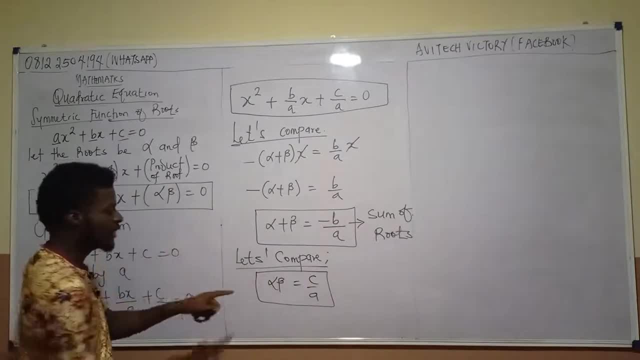 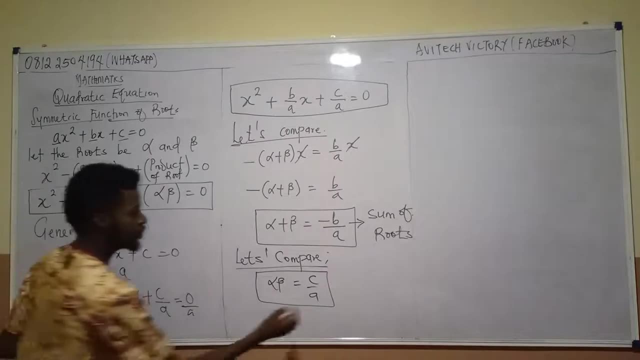 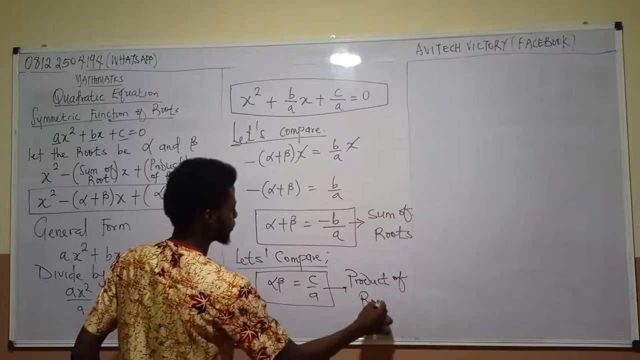 is a relationship showing that when you multiply the root of an equation, the answer is always c over a. that's the meaning. so this relationship goes for product, goes for product of roots. so the first two products i want to take down is alpha plus beta is equal minus b over a. 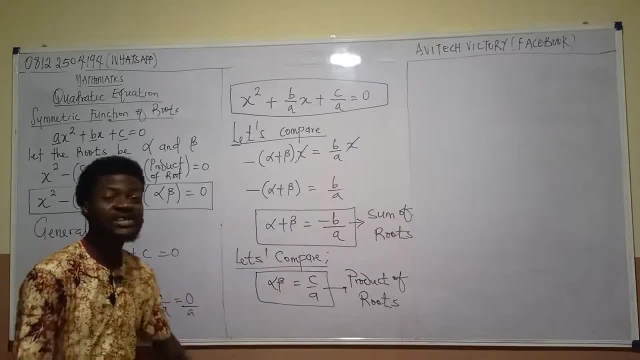 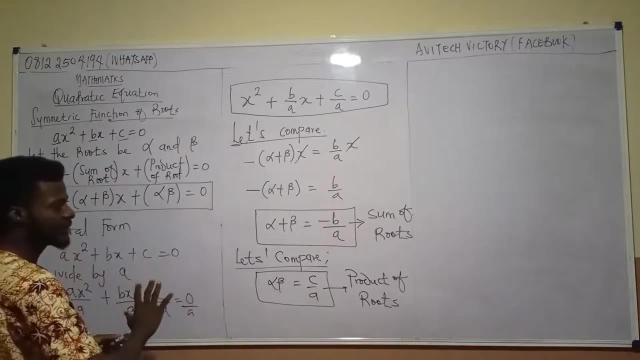 alpha beta is equal c over a. that's the first thing i want you to take. take it down, that's the first thing. um, it's not a must for you to cram how i derived it, but also try to understand it. try to understand it. but you see, these two guys. 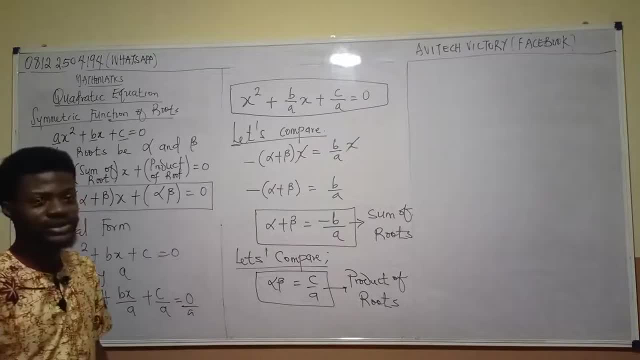 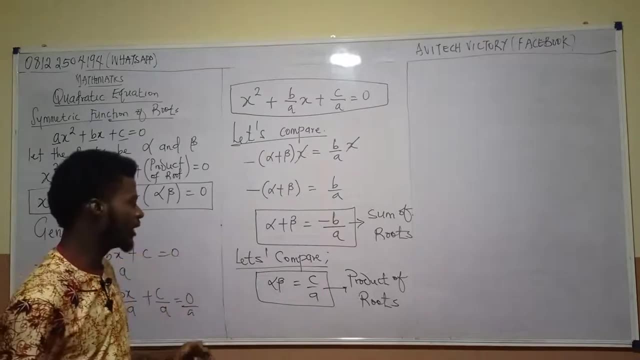 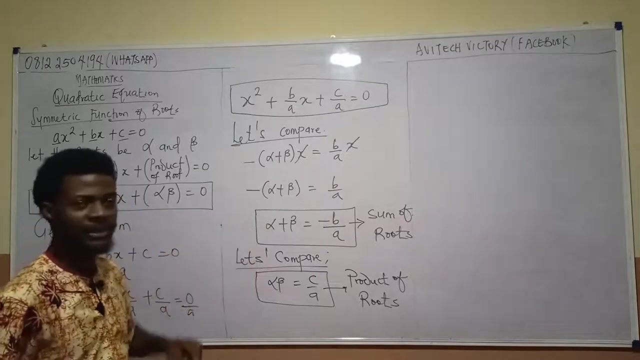 try to do it. understand it okay? so, if these two have been established, i'm going to give you formulas later on. we're going to do so many other things, but let us do one first simple equation concerning alpha plus beta and alpha beta. let us see how the equations are. let us see. 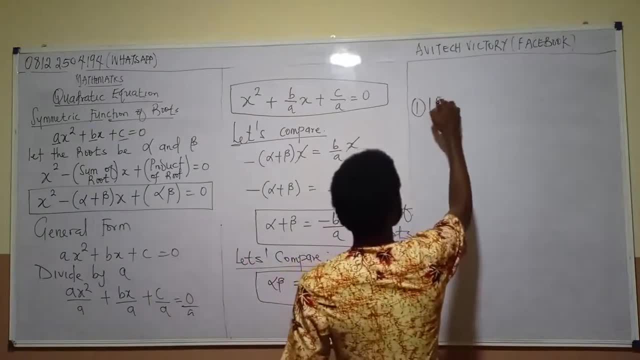 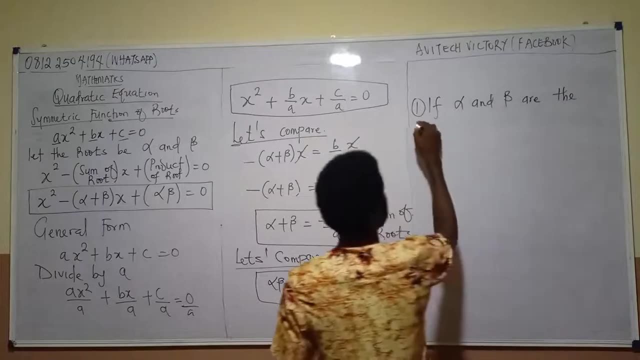 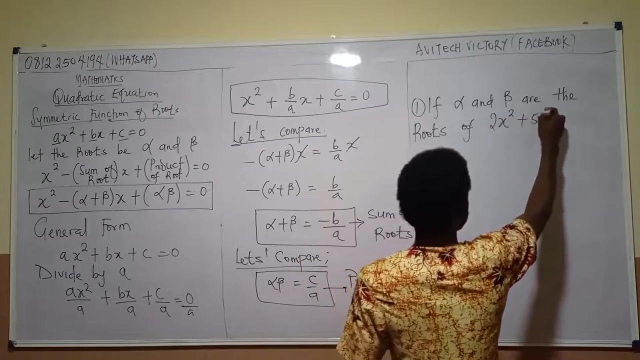 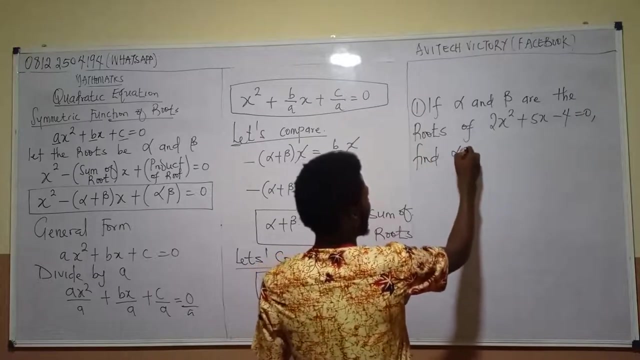 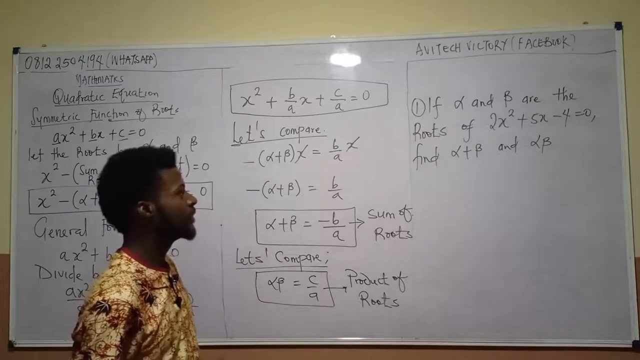 so the first question goes like this: if alpha and beta are the roots, are the roots of 2x squared plus 5x minus 4, equal to 0 comma- find alpha plus beta and alpha beta. so we have two questions there. the first one says find alpha plus beta. second one says find alpha beta. well, it's quite simple. 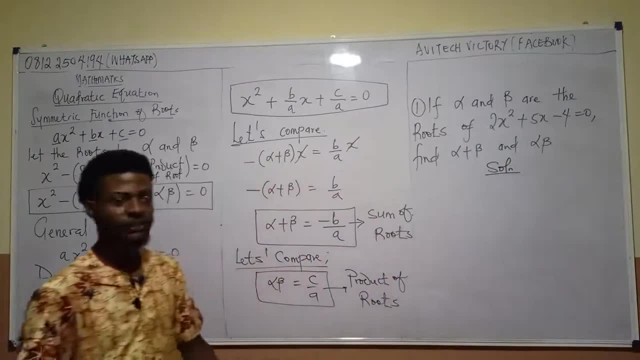 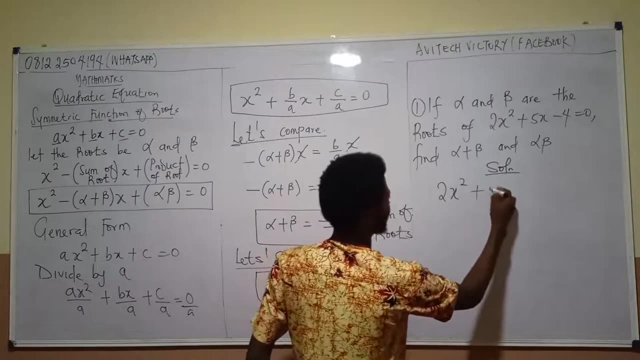 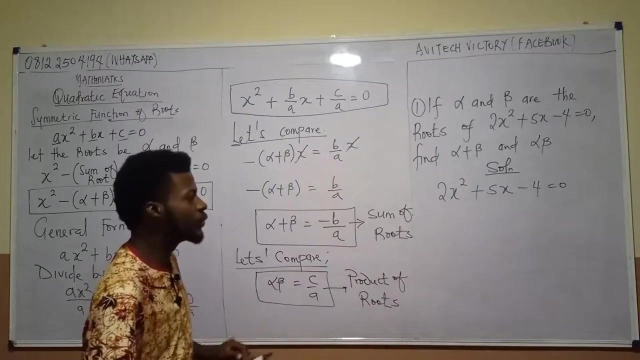 if you should have this in your exam. it's a very simple thing now, so you will do. the first thing you will do is this: you write your 2s squared, then you put plus 5x, minus 4, equal to 0. write the equation out now. it will be the first thing you will do now. the next thing you will do will be say: 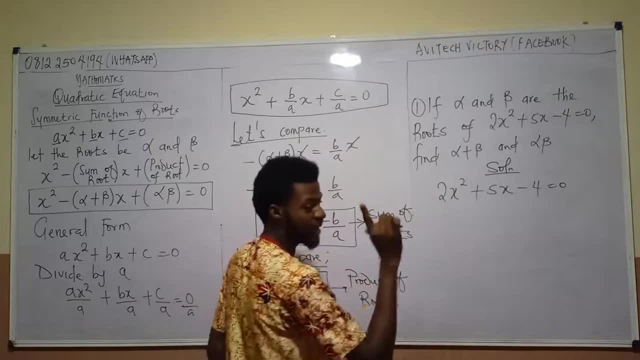 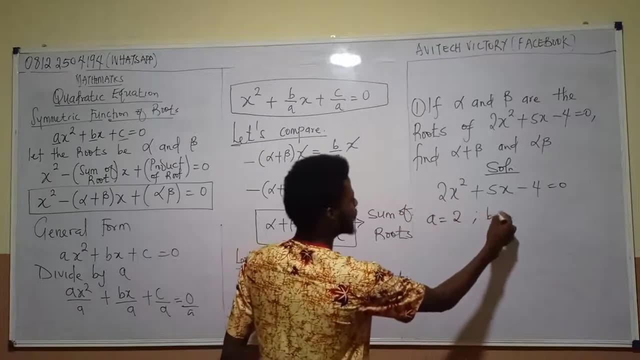 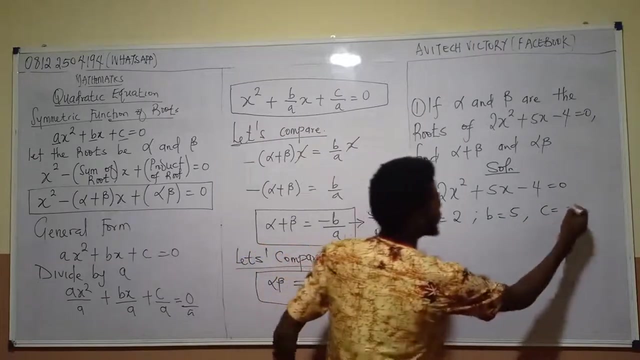 this: remember that abc, there are numbers. abc. a is the number with s squared, so what's that number 2? b is the number with x, so what's that number? 5, then c is the number we all do alone. you don't get s at last round, so that's, minus waiting, 4. now, if you don't bring out your a, bring out your b. 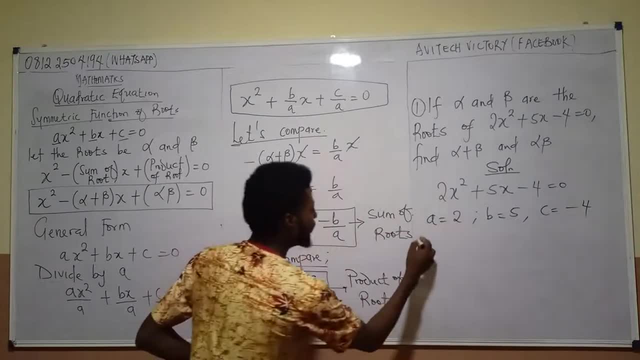 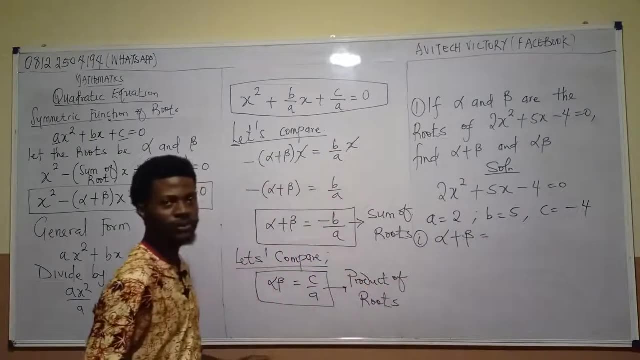 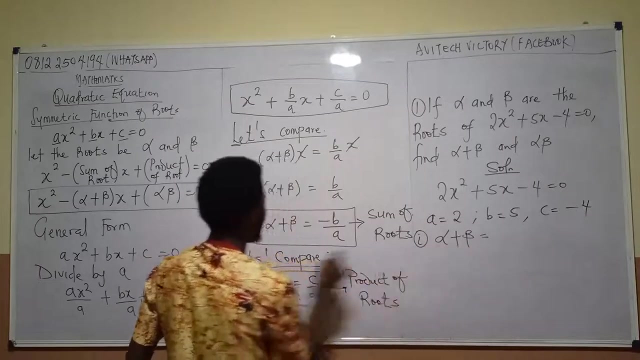 bring out your c. let us now go to the question, the first part of the question. i says: find alpha plus beta. now it's that first part top. now, since this first part has said find alpha plus beta. you don't remember the formula for alpha plus beta. so what's alpha plus beta? it's minus b over a, so you come and say minus b. 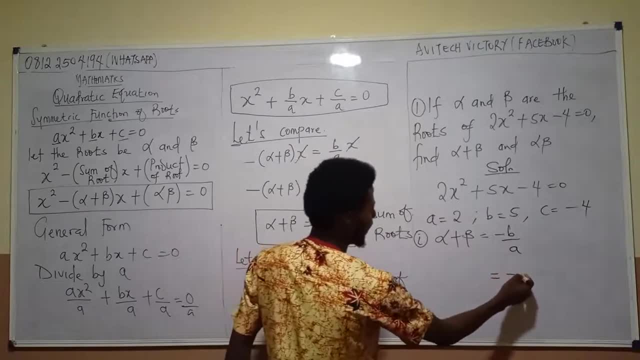 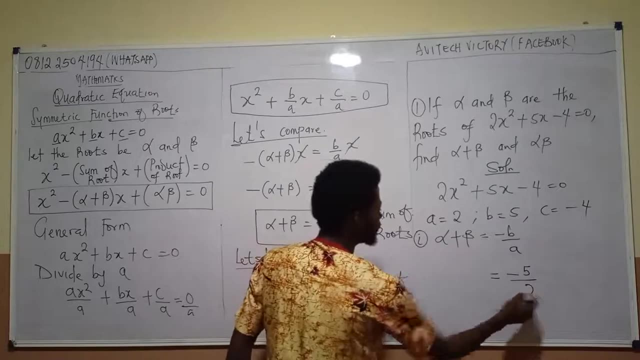 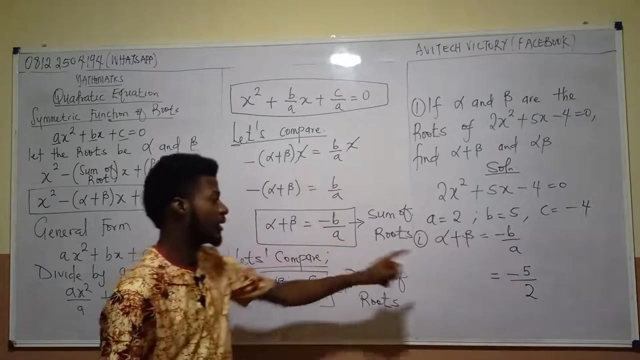 over what a. so this will be equal to minus what is b. in the question b is 5 over what is a. it's called the word 2. so that means alpha plus beta is minus b over 2. sorry, minus 5 over 2. that's the. 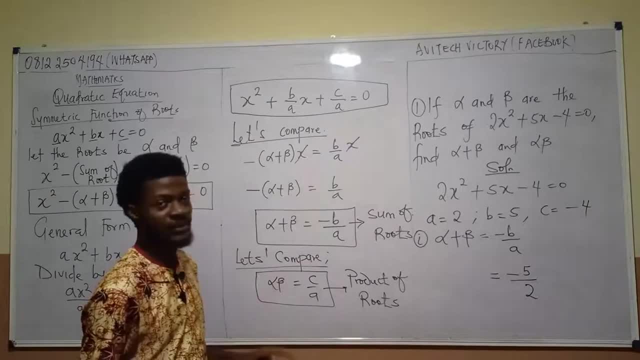 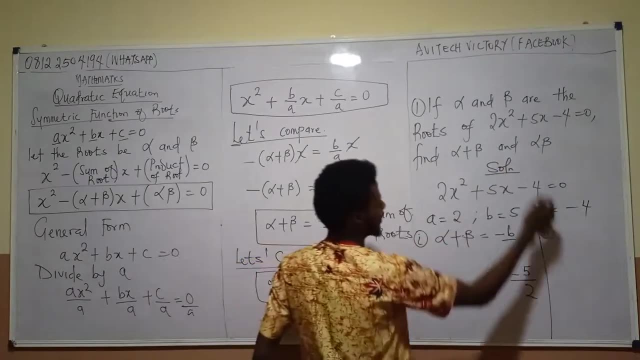 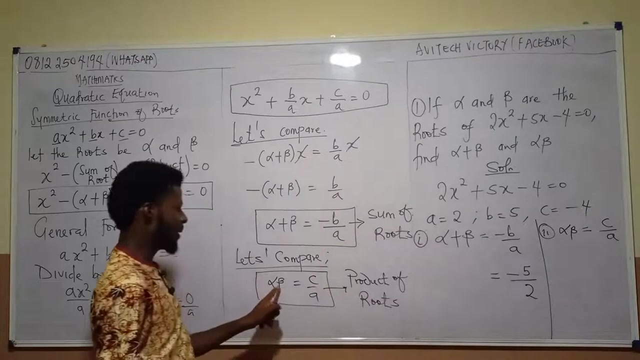 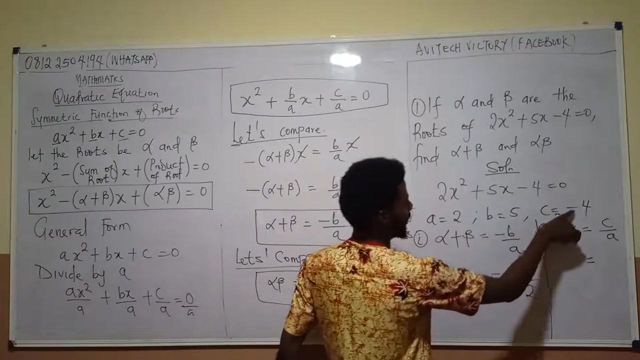 so that's what alpha is. alpha plus beta is now. the next thing is: let us look at the second part i. i let me just quickly do it here. the second part says alpha beta. alpha beta is the product of the roots and the formula is c over a. look at it. alpha beta is c over what a. so you then come and say: this is c is what minus. 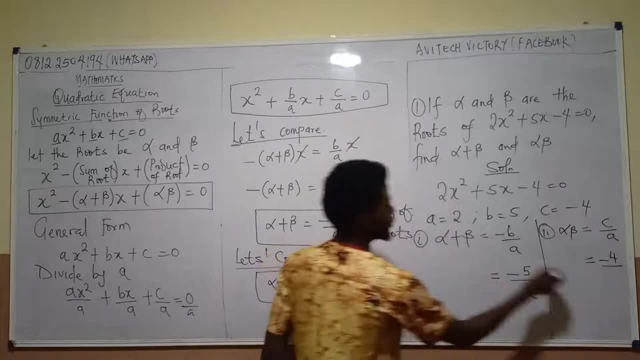 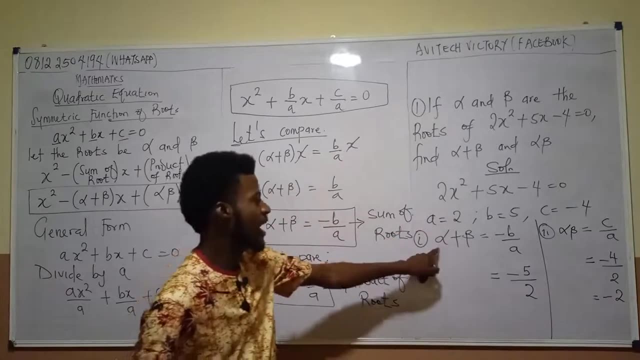 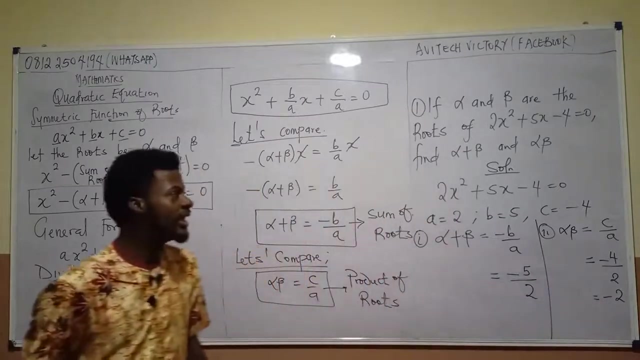 four over a is what a is two. so what's minus four over two? that'll give us what minus two. so that means alpha plus beta is minus five over two. why alpha beta is minus two. so in the course of this study i want to take note of these two things. i'm going to give you other identities to solve the